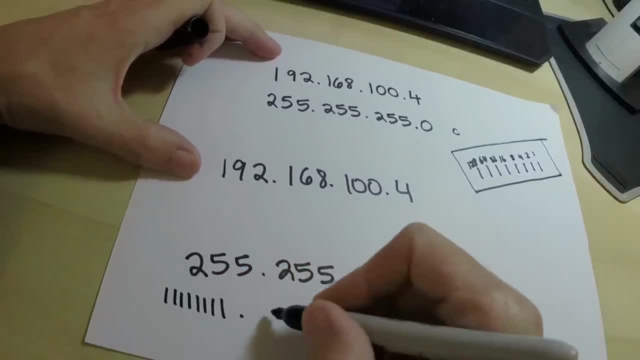 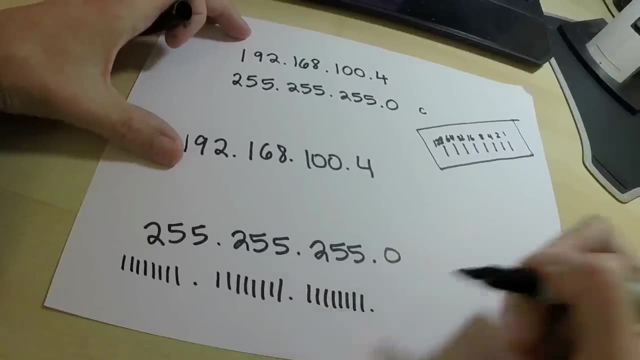 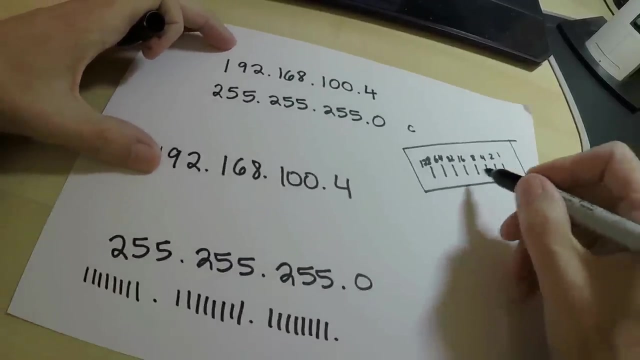 have 8 bits there maxed out. 8 bits there maxed out for 255.. 8 bits there maxed out. Now we also know this is a zero, so it can't even have a 1 here, as in the first byte. So 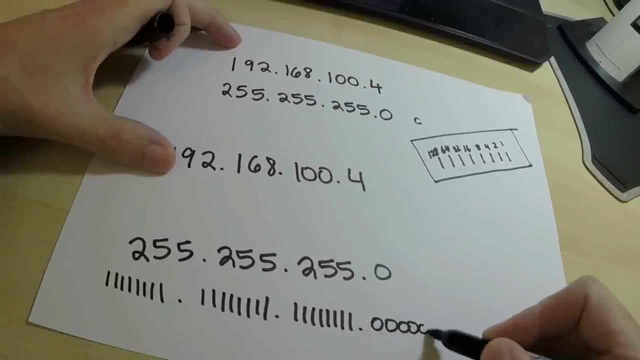 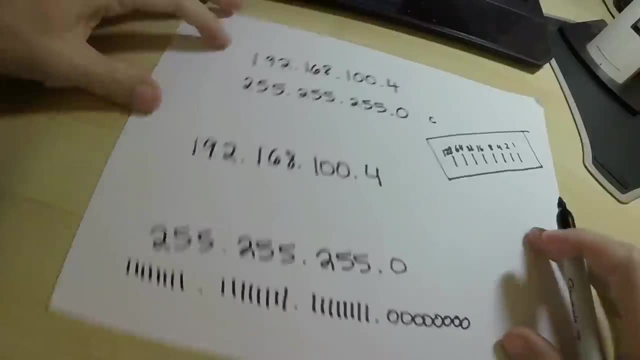 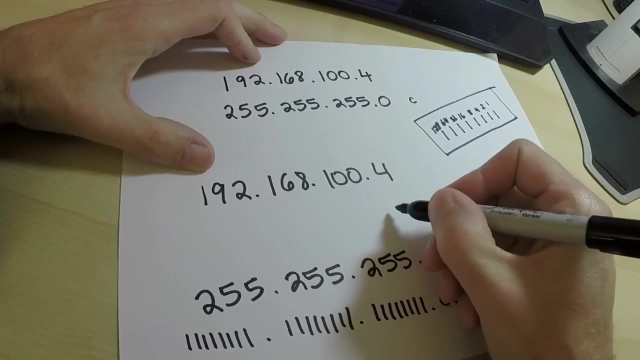 All of these would have to be 0 to represent that 7, 8.. So this is the binary representation of this netmask. Now let's do the IP, which can be a little more tricky. We'll start at the back here for number 4, and we know that the 4 is the third byte in. 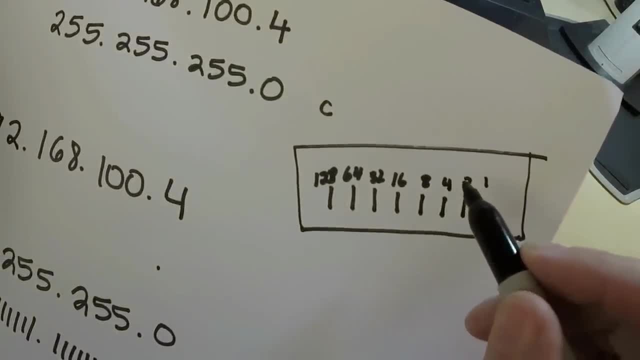 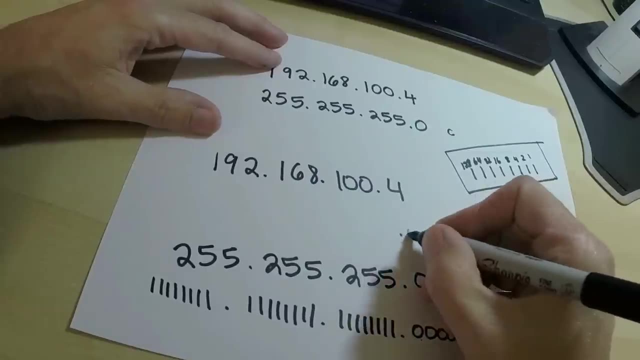 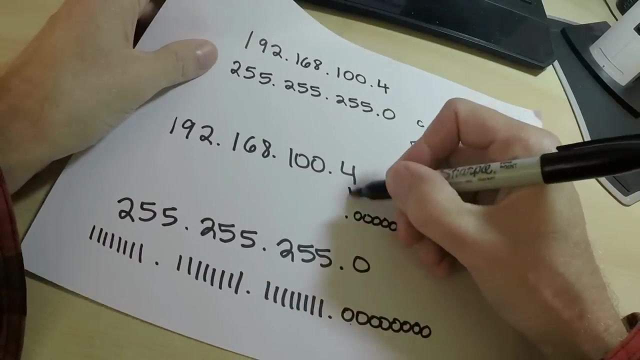 here. So we only want a 1 to count the 4, and all the others should be 0. So let's do a 1,, 2,, 3,, 4,, 5.. So we're going to do 5 zeros, a 1, and a 00, representing 4.. 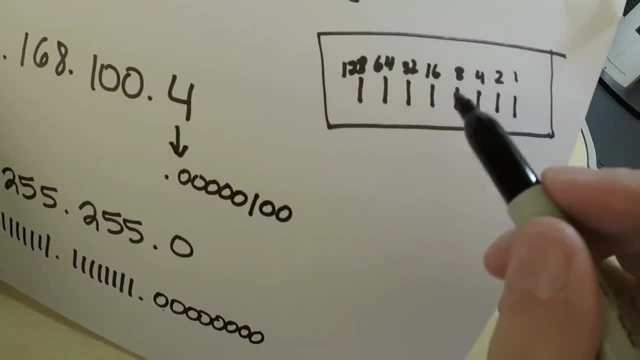 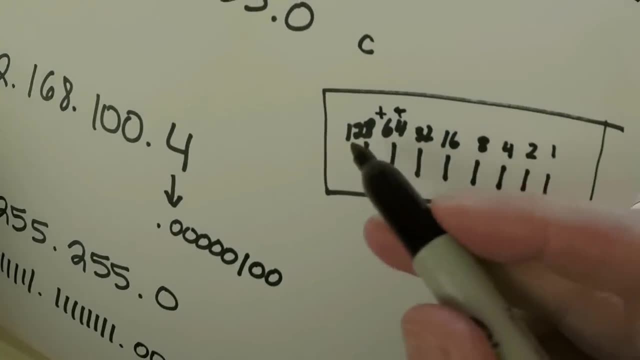 See that. And if you don't see that, what I did was say you're going to put a little 1 here for every number you want to count and there's like little plus symbols between each of these numbers across. Say, how are we going to get to 4?? 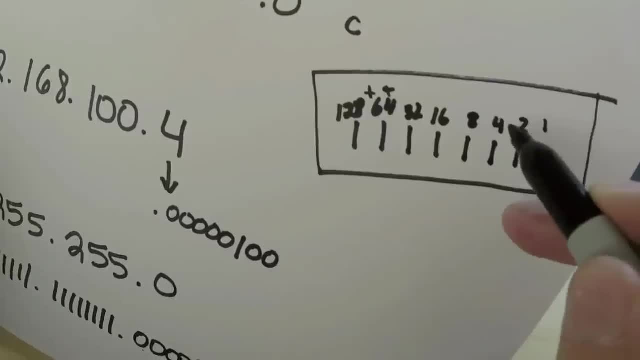 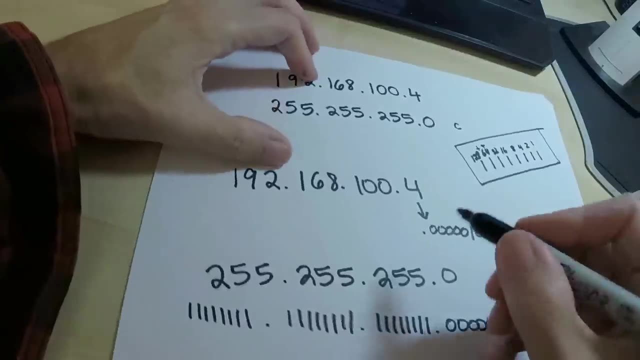 Well, we'll use this 4.. This digit right here represents a 4. We don't want to add any of these others, so they're all going to be zeros. So that is how we got this particular number. Now, let's say, we're going to find the 100.. 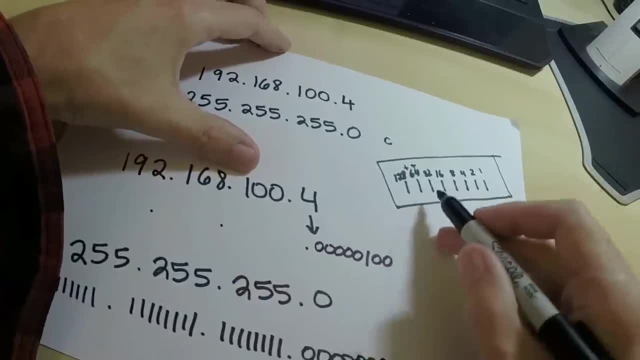 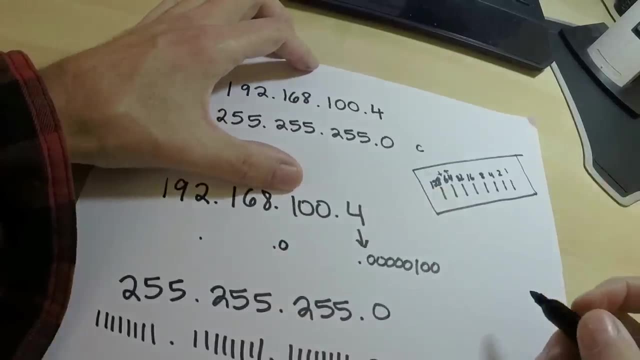 So we want to start with the greatest possible byte here. We can't use the first byte because it's 128.. We're already going to be over right, So we have to put a 0 for the first byte. Next is 64.. 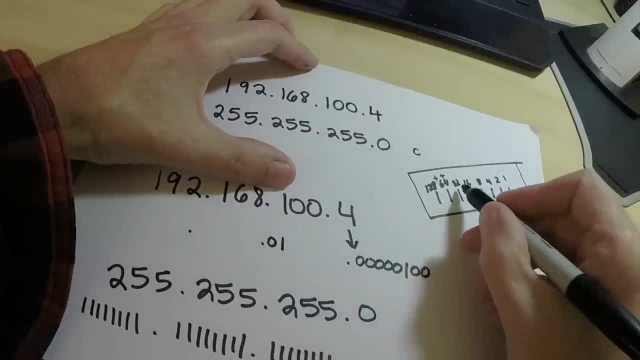 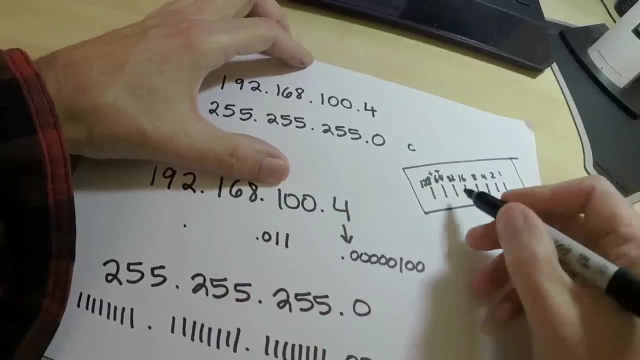 We can use that And we can also use the 32 next to it. That's going to be 96.. So we're looking for 4 more to reach the 100.. So we're going to have a 0, 0, 0 for 32,, 16, and 8.. 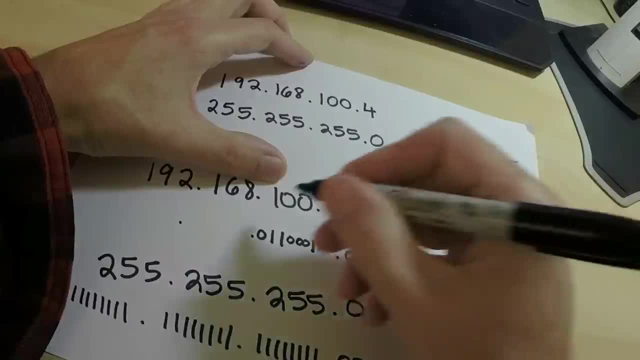 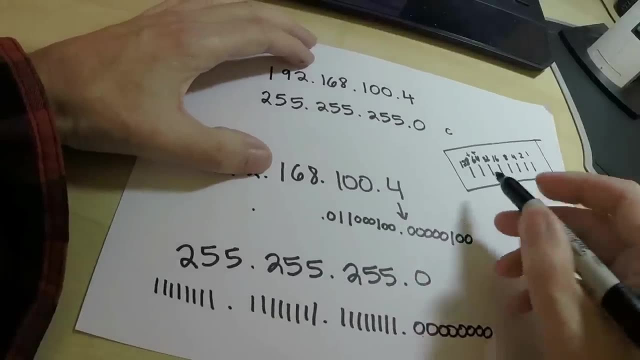 But then we come to our 4. We go, yeah, 4 is exactly what we need to finish that 100.. So the 2 and the 1 again are going to be 0.. And for the 168, the same thing again. 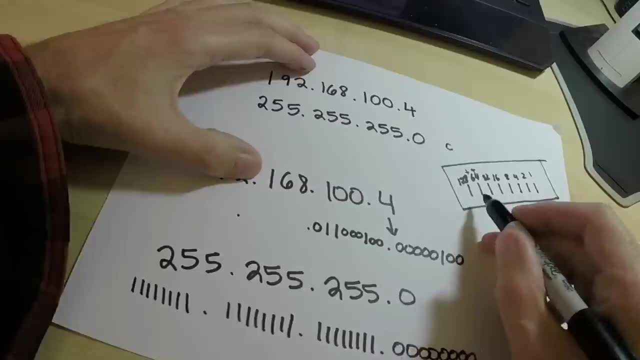 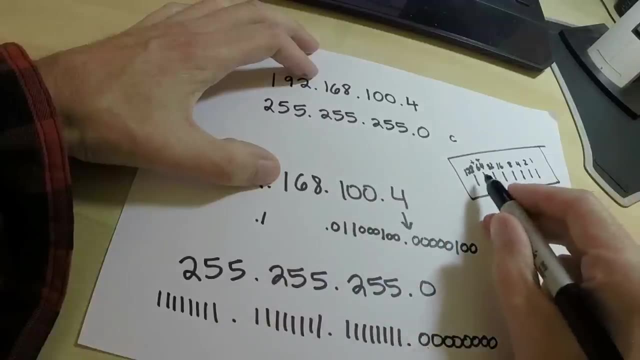 You're going to start at the most common, the most highest byte available- 128.. So we do want to put a 128 in there to start reaching this final number. We can't do 64, because that's going to put us over our number. 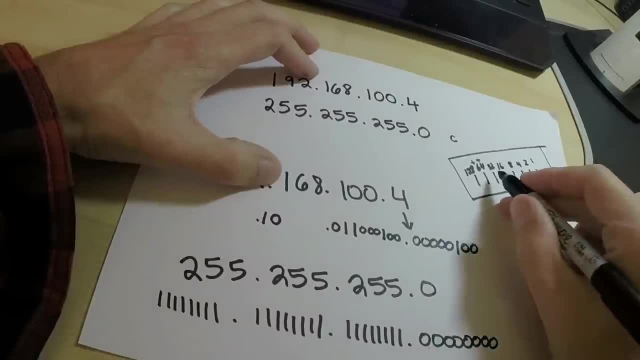 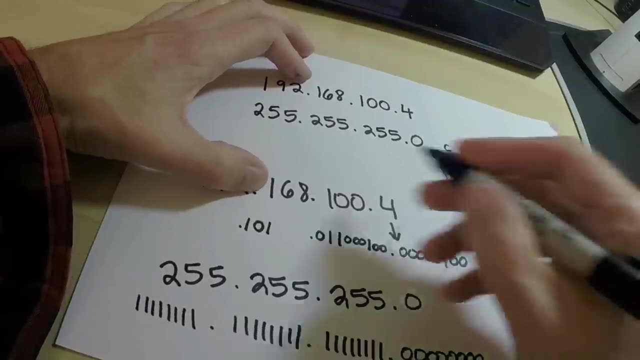 So we're going to put a 0 here. Now we can use a 32.. So let's put in a 32 here, which will give us 160.. Now you can see, we only need 8 more. So we don't want the 16.. 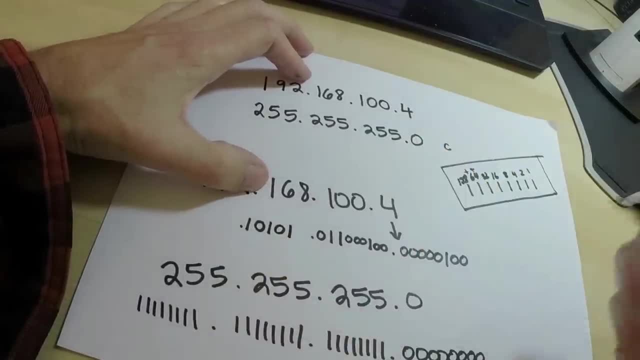 Let's 0 that out. The 8 is next. We want the 8. And there we go. That's perfect. So we don't want to use the 4,, the 2, or the 1.. 0,, 0,, 0.. 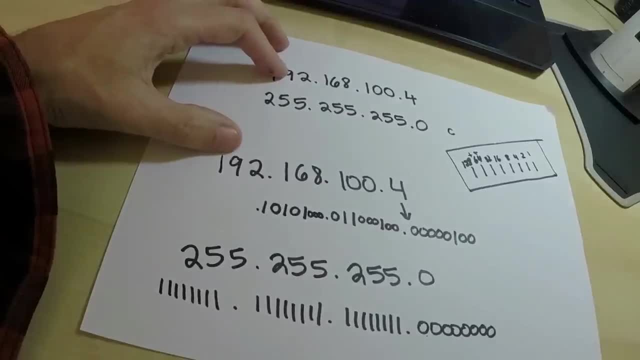 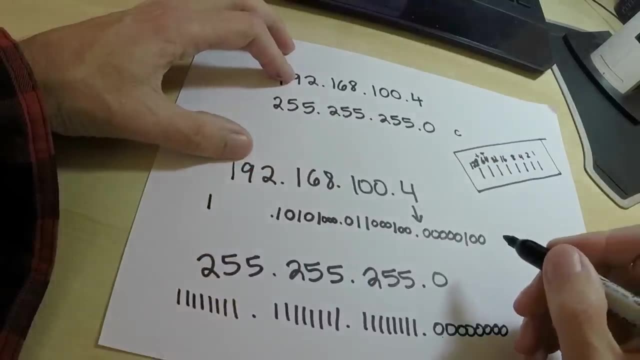 Don't use those. And for the 192, we're going to start with the largest bit, which is 128.. We're going to use that And we're also going to use the 64. And that is going to equal exactly 192. 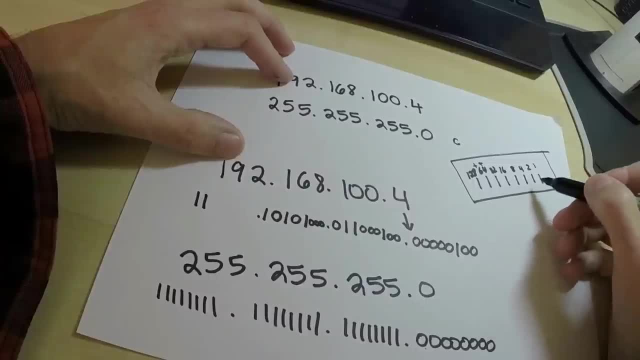 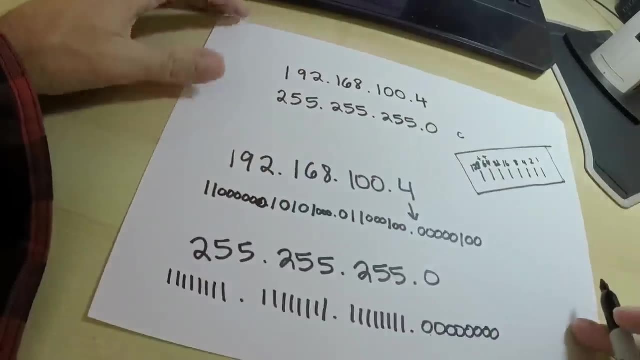 with the first two bits there, So all the others have to be 0.. We're not going to use those, So that's going to be six 0s: 1, 2, 3.. 4, 5, 6.. 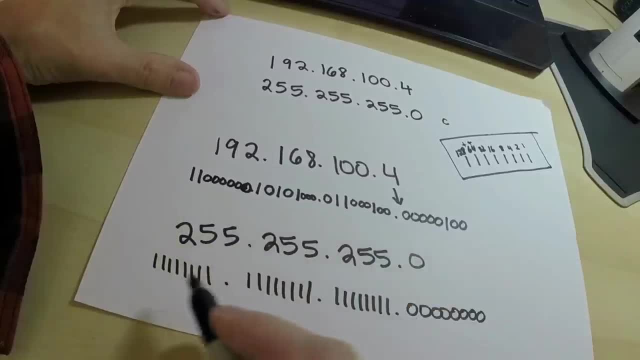 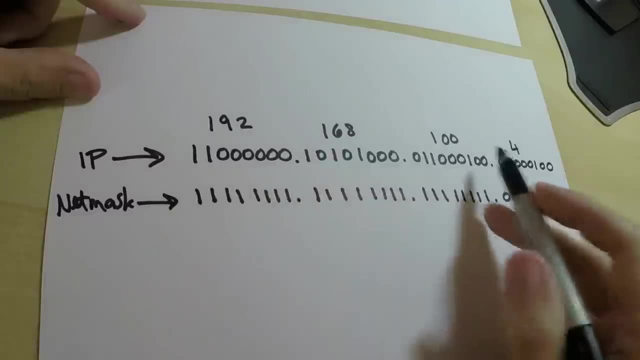 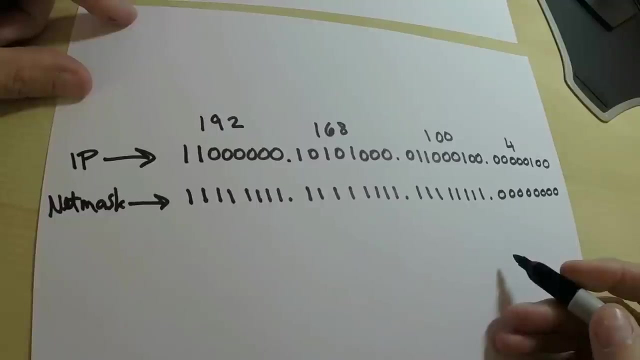 Now we have the binary representation of this IP and this netmask, All right, so I made a fresh sheet here. So again, we have our IP here and our network here. How do we find the broadcast address of this IP? So what you do is you look at the bottom netmask. 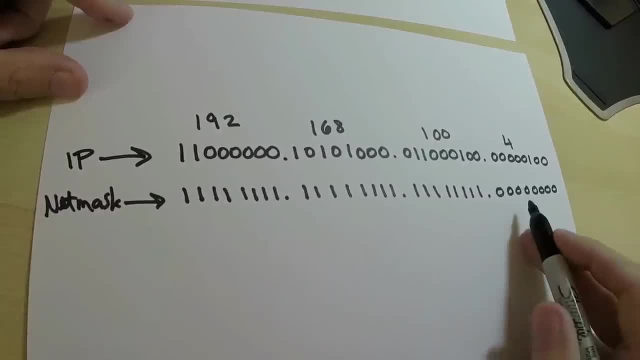 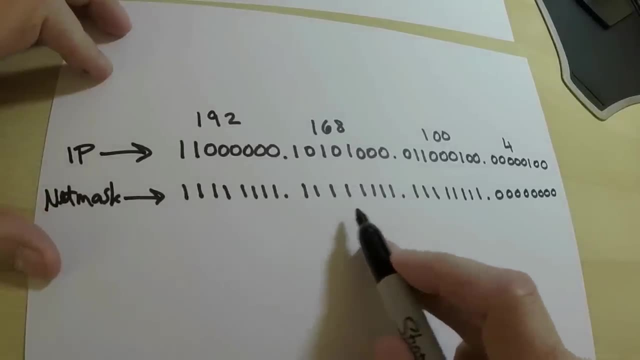 And whenever the bottom netmask value is 0, you have to change the above section. You have to change the above section to a 1.. So let's go ahead and go through here. No 0s, no 0s, no 0s. 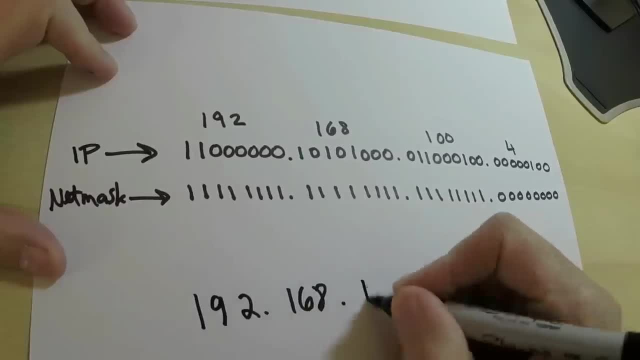 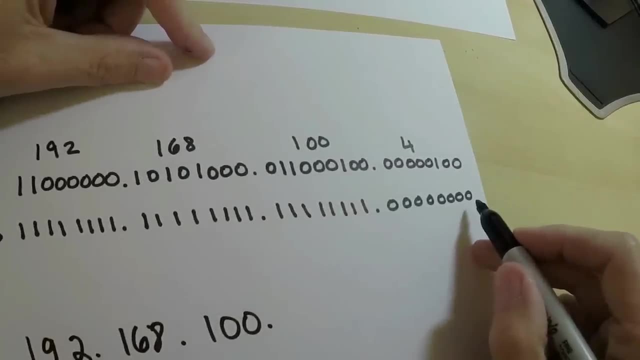 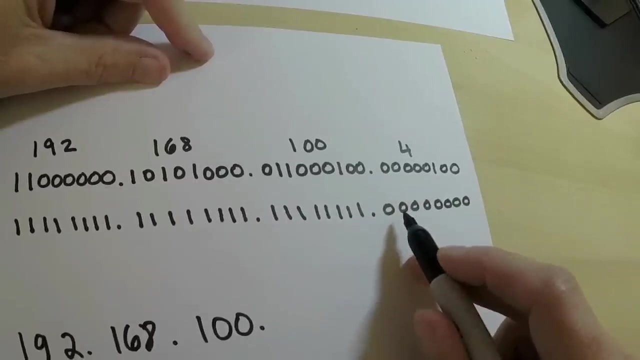 So this part is not going to change, But over here we have some work to do. This is all 0s. So what this means is that everything above it is going to have to change to a 1.. So any time you have a 0 in the bottom netmask. 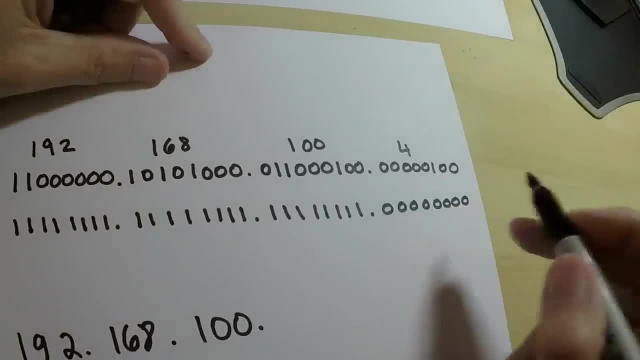 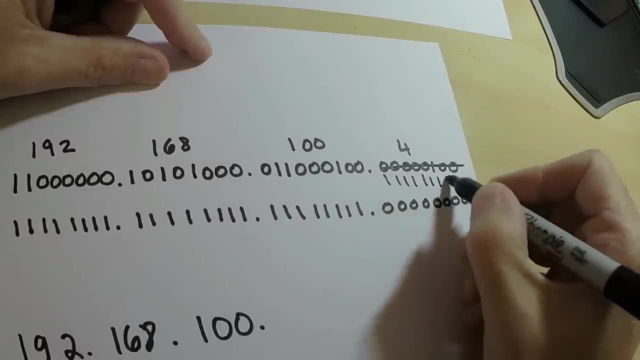 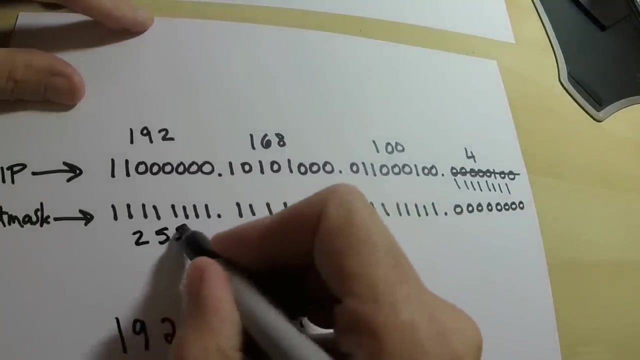 that means change the above section. That means change the ones above it to a 1.. This is all 0s, So we have to change this to all 1s And, as we know, all 1s equals a 255, as we've seen here.